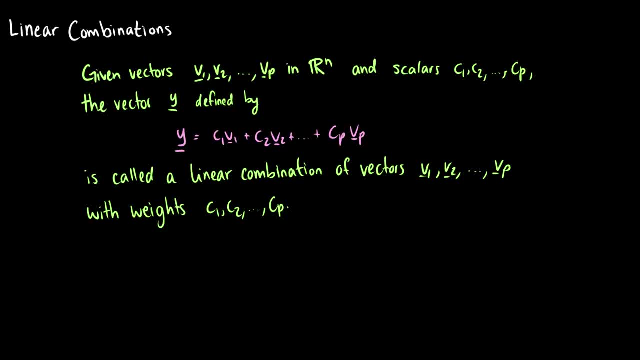 In this video we're going to talk about linear combinations, So we're going to get a little bit more notation heavy and into general concepts. So what is a linear combination? Given some vectors, v1 through vp in the real numbers and scalars, c1 through cp, we define a vector y as c1 times v1. 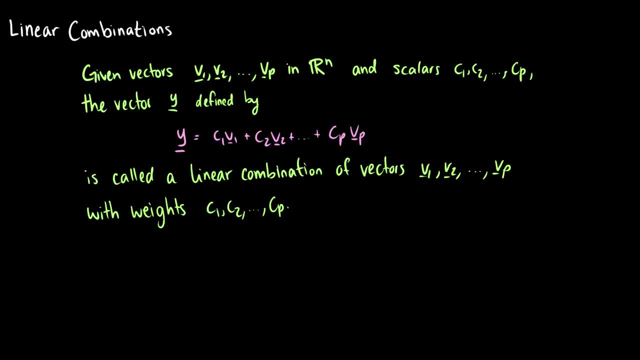 plus c2 times v2 plus cp times vp. This is a linear combination with vectors v1 through vp, with weights c1 through cp. So what does this look like? What's an example? Let's say y is equal to 3 times the vector a1 plus 2 times the vector a2.. That is an example of a linear. 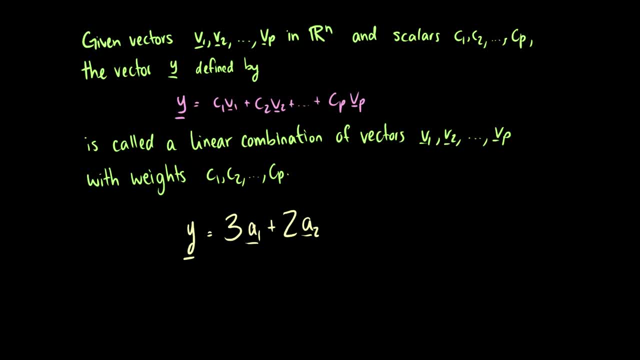 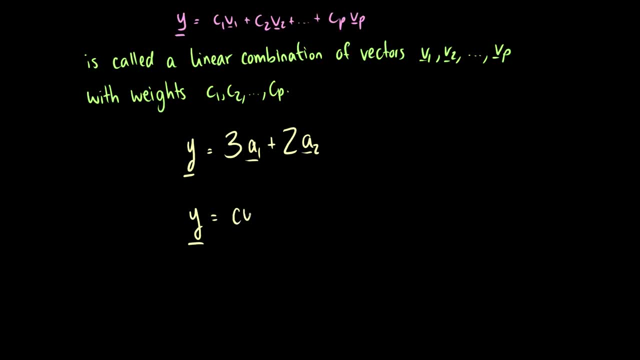 combination, Or perhaps in the previous video you might have seen this, as y is equal to c times the vector u plus c times the vector v. So this is another way of saying a linear combination. But we just have a little bit more general variables saying okay, it's up to p scalars and p vectors. So here's an example. 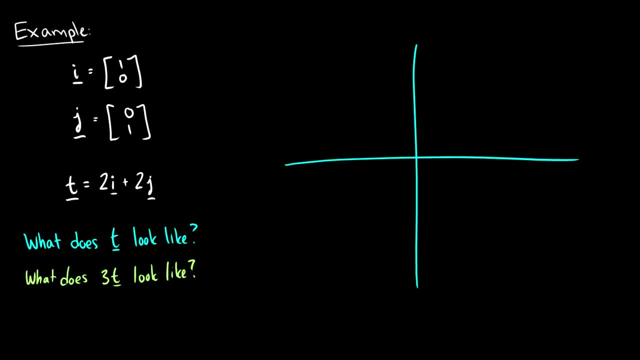 We have the vector i, which is 1,0.. So this looks kind of like this: This is the unit vector in the x1 direction, so we can call this the i plane and the j plane. So that is i. We have j going 1 towards this direction, so we'll call this j. We're saying: 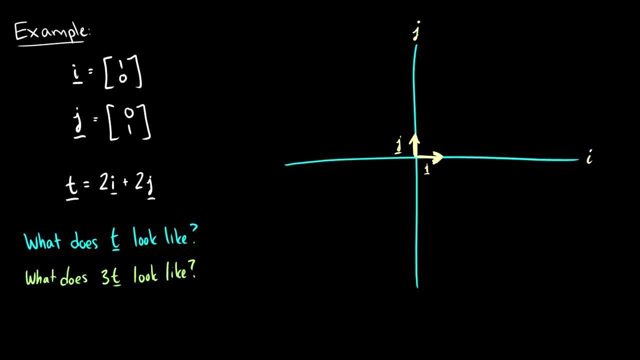 this vector, t is equal to 2 times the vector i plus 2 times the vector j. So let's take another i, and let's take another j, And where do we end up? Well, we end up at this point here. So t is this vector, This is t And t is just a linear. 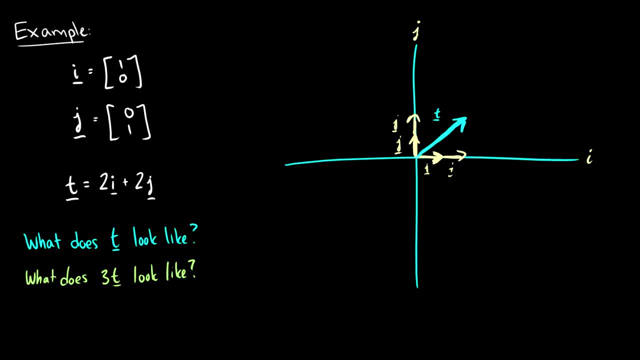 combination of i and j. So t looks like an arrow going up to the right, And we just made a combination of two unit vectors to get there. So what does 3t look like? Well, if we take t, we can do two more t's and then we get this big vector which is 3t. And what if we didn't want to call? 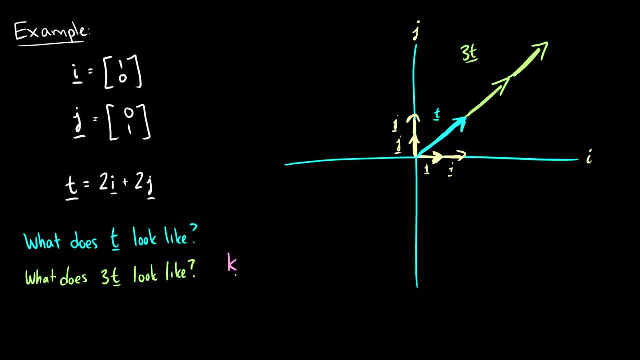 this 3t. We could say: okay, well, vector k is just equal to 3 times the vector t, which in itself is just 6i plus 6j. But we've used the linear combinations of i and j to get a vector k, So k here. 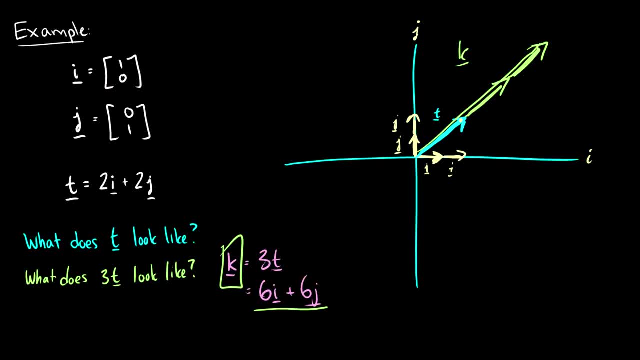 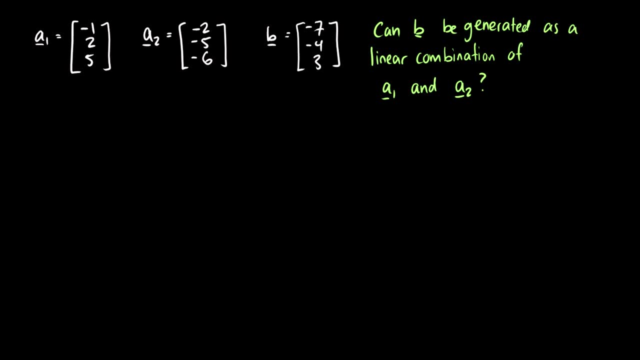 the linear combination of vectors i and j. So that is what a linear combination is. So here's a question: We can ask if some vector b can be generated by a linear combination of a one and a two. So this question is saying: okay. 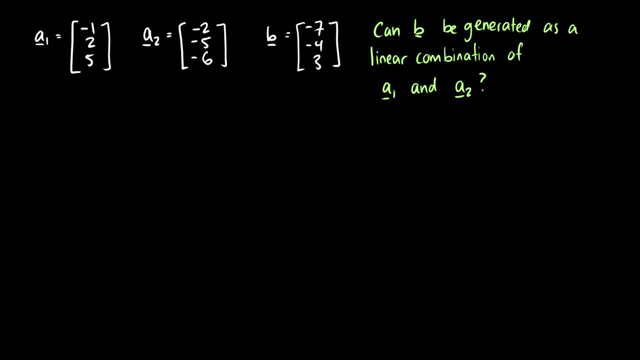 is it possible to get this vector negative seven, negative four, three, by having some number of a's, a ones, and having some number of a twos. Well, we can solve this. So what we can do is we can put a one, a two. 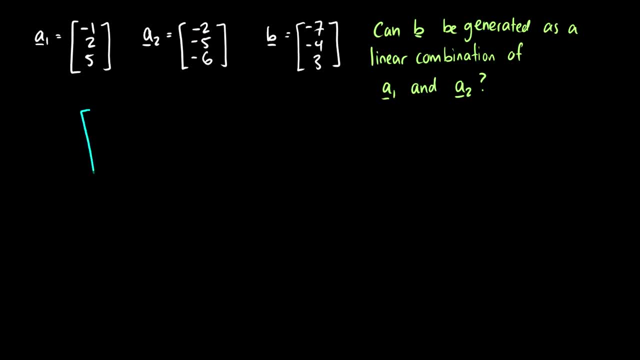 and b into a matrix. We can say: okay, we have negative one, two, five negative two, negative five, negative six and negative seven, negative four, three, and we can solve for this. Why can we do this? 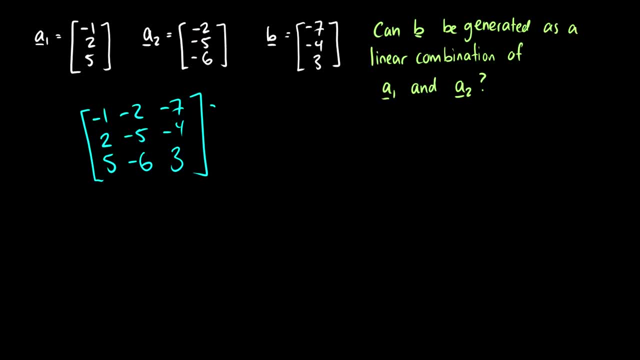 Well, when we do this, we can multiply by x one and x two and figure out values for x one and x two, and we're good, But we're going to cover this more specifically in another video. So we want to see how many of the first row 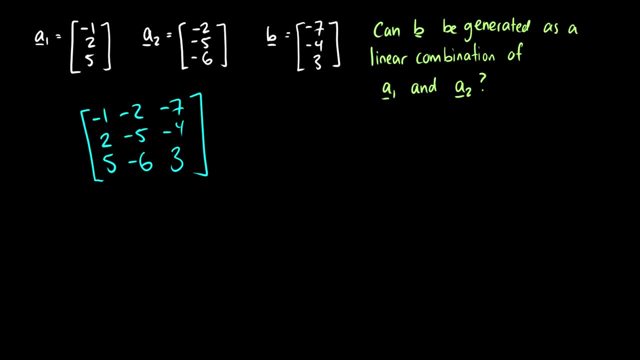 or sorry, the first column plus how many of the second column get to the third column. So let's just reduce this and we'll see what happens as we go. So let's multiply the first row by negative one, because I don't like dealing with negative numbers. 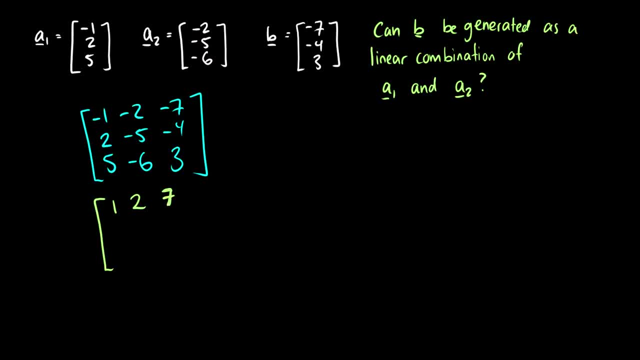 They're a little bit more confusing, a little bit more problematic, They're prone to make mistakes And for the second row we're going to take two minus the second row. So it's going to be the second row minus two of the first row. 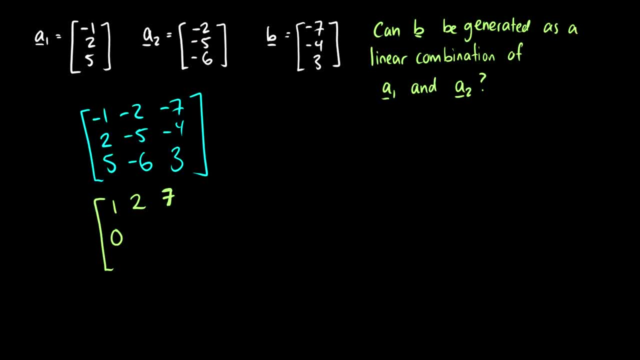 So we're going to have: two minus two is zero Negative. five minus four is negative nine. Negative. four minus 14 is negative 18.. And then we're going to take the third row minus five of the first row. So five minus five is zero. 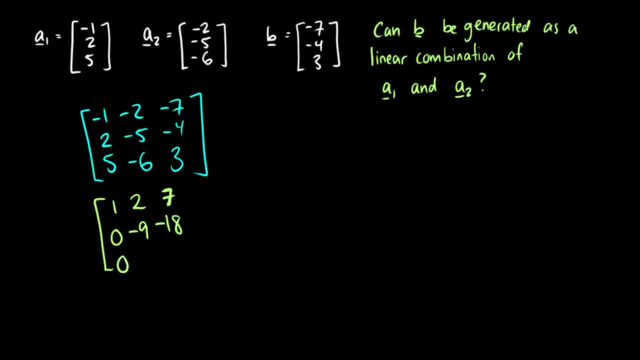 Negative six minus negative 10 is four, And three minus negative 35 is 38.. I believe I did that right, So adding five of the first row. So this should be negative 16 and this should be negative 32.. Okay, so I believe now we are good. 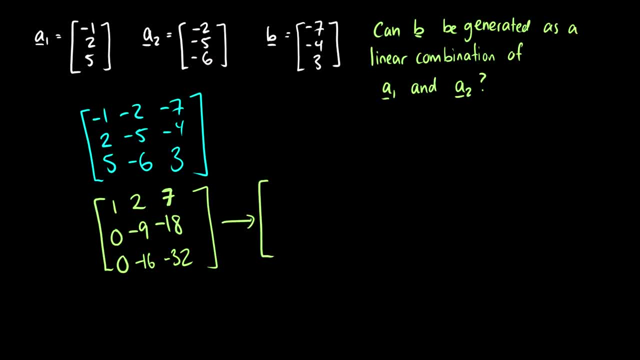 Okay, So now let's do some quick multiplication. So we have one, two, seven. Let's divide the second row by negative nine, So we're going to get zero one, two. Let's divide the third row by negative 16.. 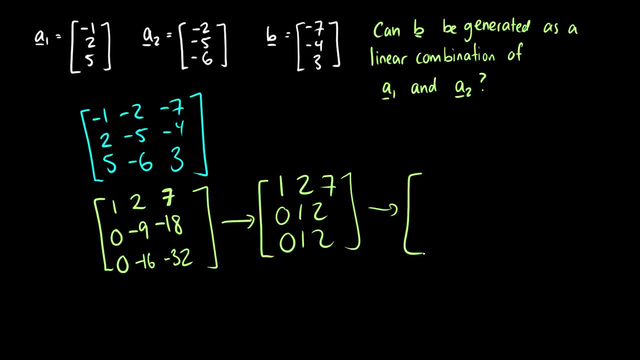 Zero one two. We can eliminate the third row because the second row is an exact copy of it. So we get zero one two, zero, zero, zero. So now we get that X two is equal to two and X one is equal to seven minus two, zero zero. 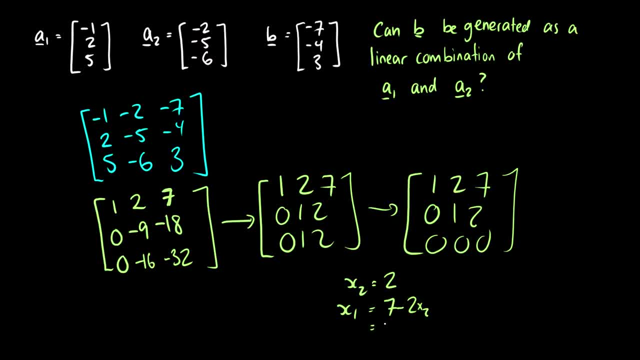 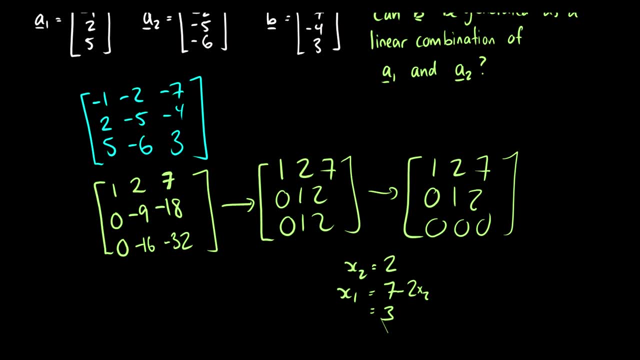 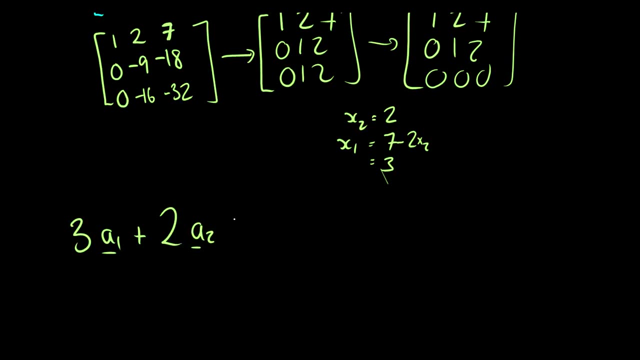 X two, which is just seven minus two times two, is four. Seven minus four is three. So we've now solved the system. So here's what we're saying. We're saying that three times A one plus two times A two is equal to B. 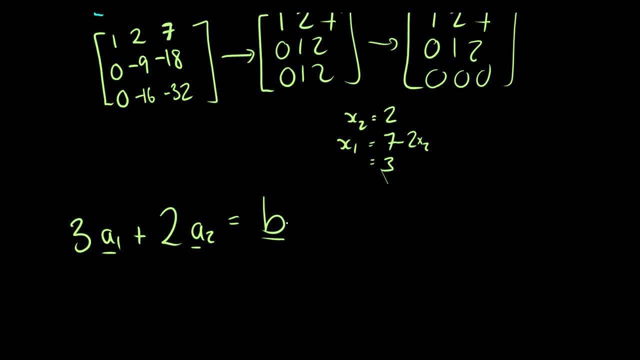 Why is this? Well, remember a linear combination B. So we have before. our definition of Y is just X one times A, one plus X, two times A, two, all the way up to plus XP times AP. Well, here we just have our X one A one. 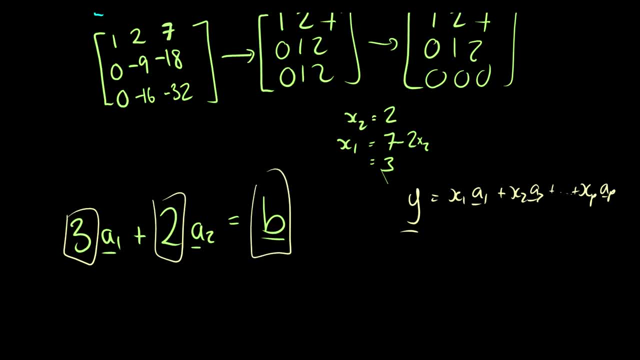 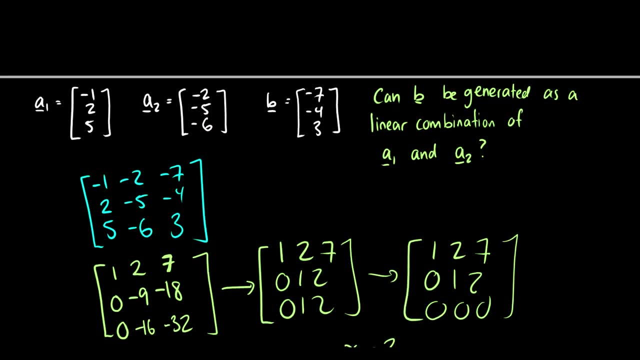 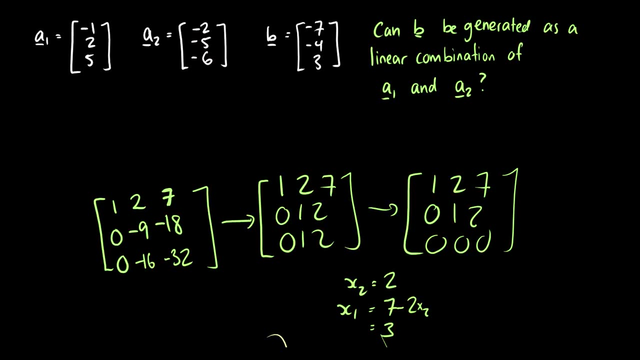 plus X, two A two is equal to our vector B. So three of the first vector plus two of the second vector makes B. Let's check to see if this is true. Okay, So let's take three A one. So this will be three times negative one, two, five. 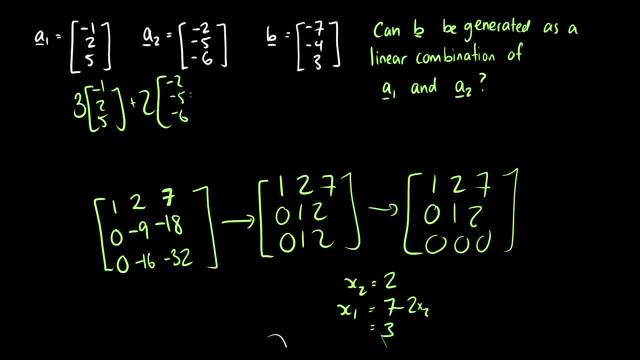 plus two times negative, two negative five negative six, And this should equal negative seven. negative four, three. Okay, So this is going to be negative three, six, 15, plus negative four. negative 10, negative 12.. 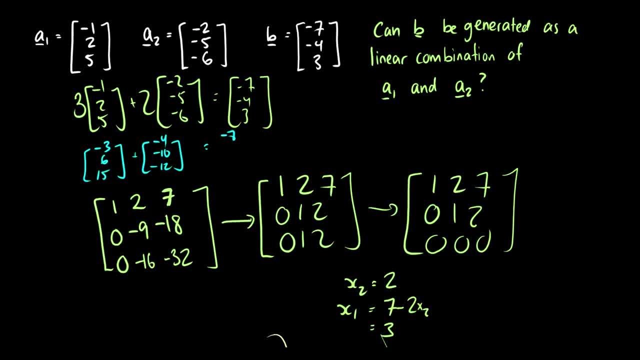 Three plus negative four is negative seven. Six minus 10 is negative four. 15 minus 12 is three. So there we go, There is our solution. So B can be generated as a linear combination of A one and A two. So if we only have vectors A one and A two in our system, 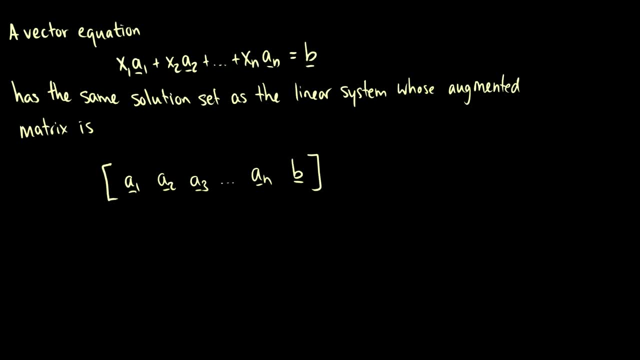 we can make vector B. So here's a vector equation: X one, A one plus X two, A two all the way up to X, and A n equals B. This has the same solution set as the linear system whose augmented matrix is A one through A, n and B. 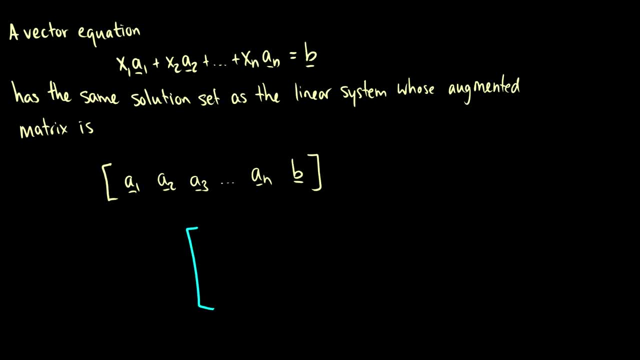 So this is the exact same thing as we did in the previous one. We said: is A one plus A two, can this linear combination generate B? So we solve the matrix and we found out that yes, it can. So when I say these vectors, A one in the system, 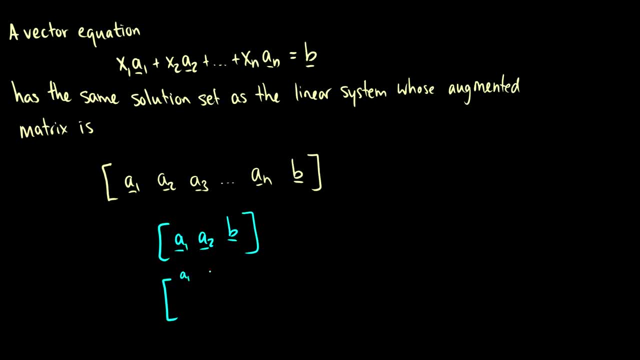 what I really mean is we have- okay, we have, you know this- a11 all the way down to am1, so that's the first line. Then we have a12 all the way down to am2, and then we have b1 all the way down to bm. So this is just short form for the whole vector. 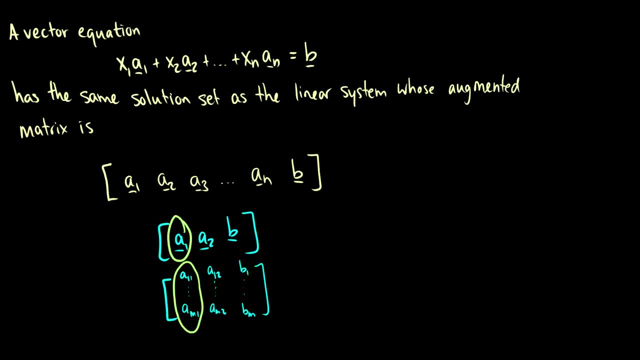 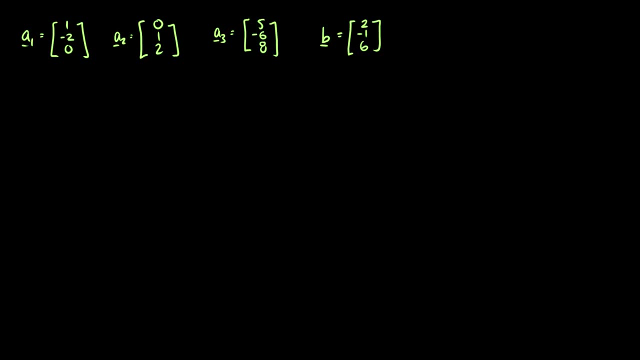 so these two are exactly the same. So with this we were able to solve the question and figure out that b was a linear combination of a1 and a2.. So again, let's do this. again, We want to find if b is a linear combination of a1, a2, and a3. So we're going to stick these all into a matrix. 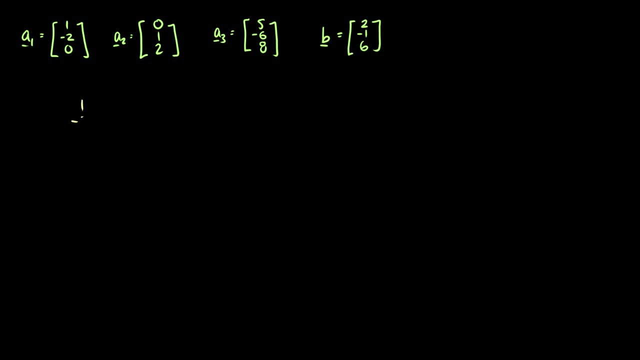 I'm going to use a different color. so 1, negative, 2, 0, 0, 1, 2, 5, negative, 6, 8.. Do these generate 2, negative, 1, 6?? So what we can do is we can look at it. 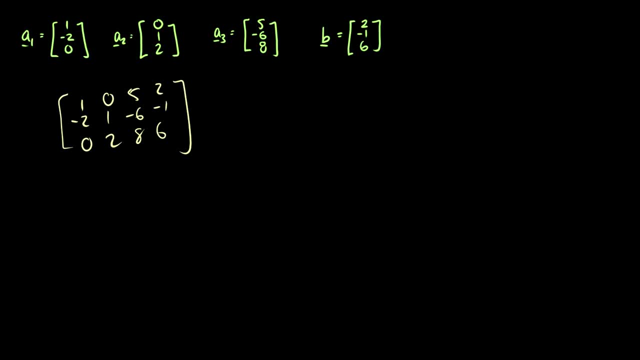 and figure it out in our heads. if we want to, We can say: well, it looks like if we take 1 of a3, and we subtract 3 of a1, and do something with a2,, maybe we can get it, but probably best to. 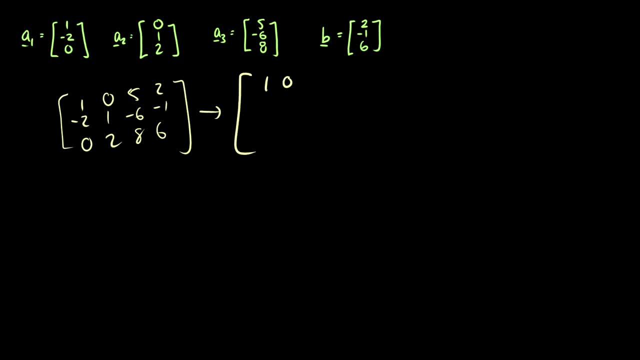 solve it. So let's keep row 1 the same. We're going to divide row 3 by 2, because it looks a little bit messy, And let's take a look at row 2 here. So we want to add 2 of row 1.. So we're. 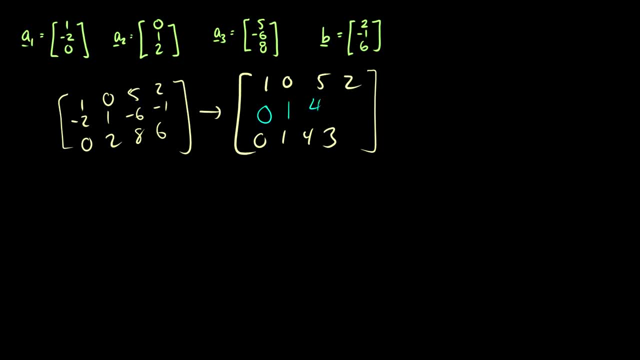 going to get 0, 1, 4.. We're going to add 2 of row 1, 3.. Oh, look at this. Our second and third rows are exactly the same, So we can look at this and we can just delete the third row. 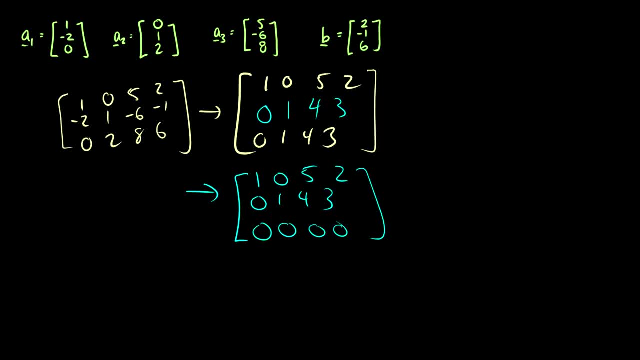 Okay. so what do we have here? Well, we have this system with a free variable in it. This says that x1 plus 5x3 is equal to 2, and x2 plus 4x3 is equal to 3.. So again, 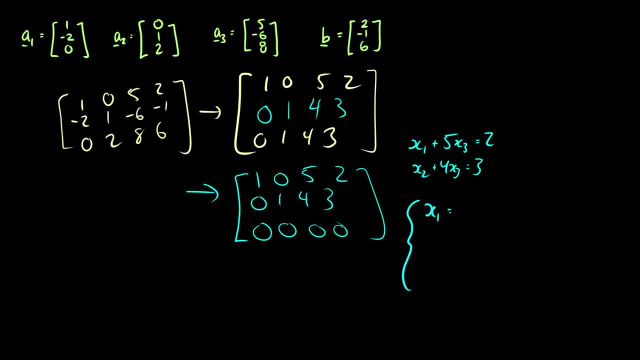 we have this solution set: x1 is equal to 2 minus 5x3.. x2 is equal to 3 minus 4x3. And x3 is free. So this is a solution set. So, yeah, b can be generated with x1,, x2, and x3.. We have to give a certain value for x3,. 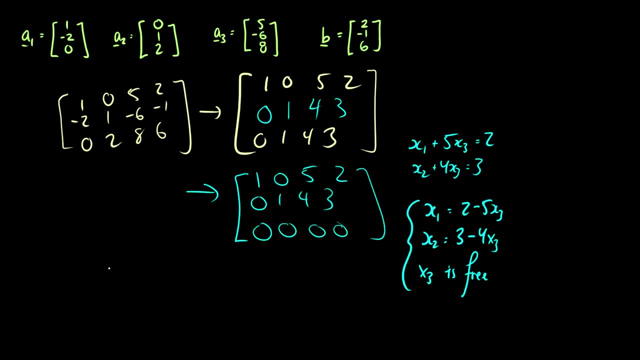 so we can find one solution. We can say: okay, suppose x3 is equal to 0. And that means that x2 is equal to 3, and x1 is equal to 2.. So now we can say that, yeah, so 2a1 plus 3 of a2 will. 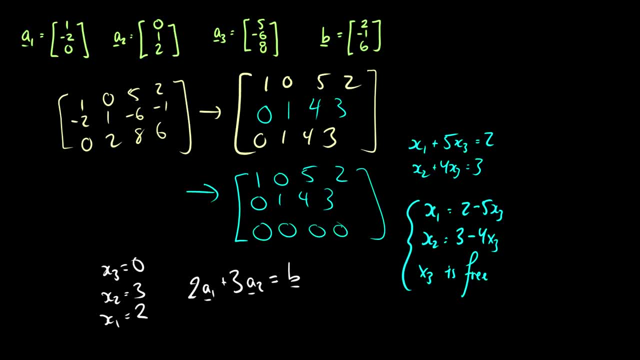 give you b. So that's one solution We can pick. x3 is equal to 1, and we can get a different solution. So there's many different ways. we can use x1,, x2, and x3, or, sorry, we can use a1,, a2, and a3 to get the vector b. 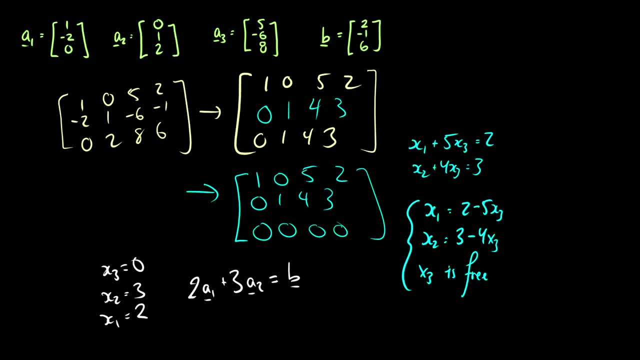 In fact in this first, if we pick, x3 is equal to 0, we don't even need x1 and x2.. I mean, we don't even need a3 at all, We can just use a1 and a2..